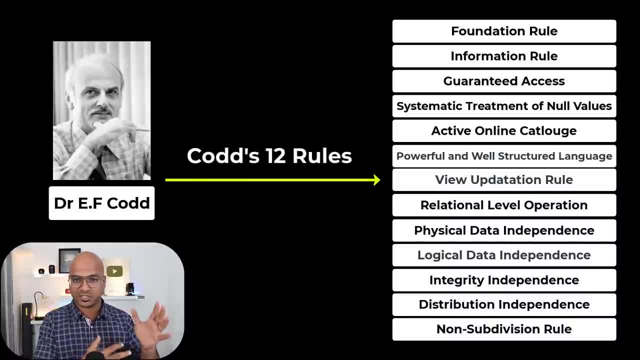 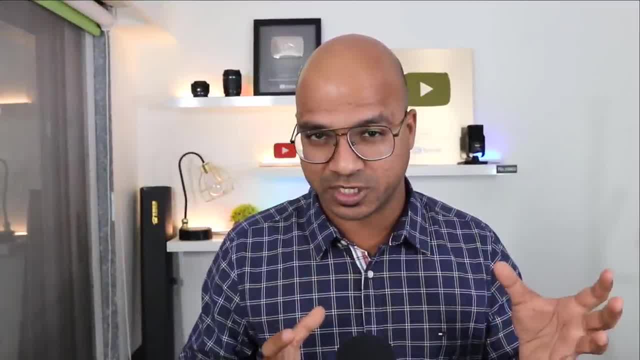 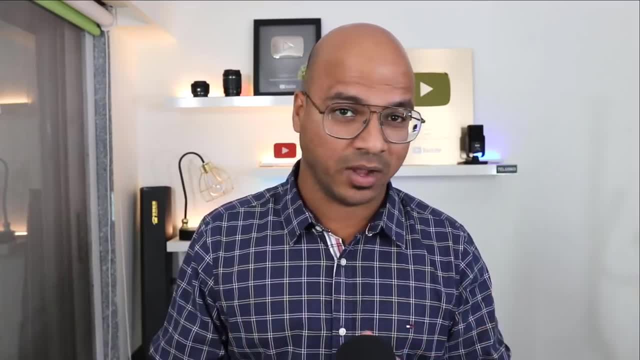 this tool rules based on which we got this database system right, and that was relational database, basically where you have tables right, you have multiple tables which are related to each other. the actual term of relation came from something else, from maths, but let's keep it there. we have multiple tables and they are related, right, so there were primary keys, foreign keys and 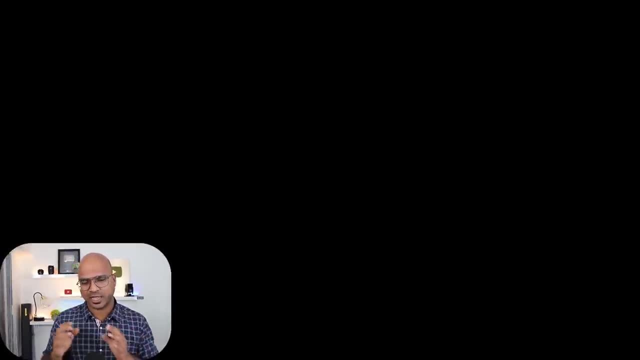 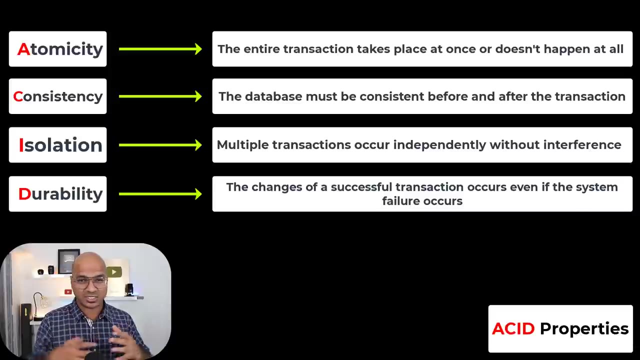 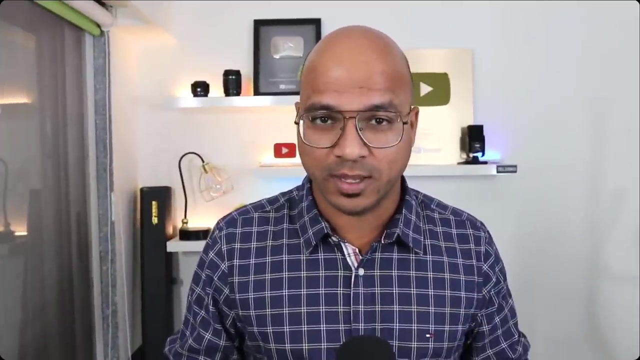 different stuff right now. the basic idea of relational database is it actually provides you something called asset properties, right, which is this is asset property. it provides you consistency, durability and all those stuff and important stuff, right? for example, let's say, if you do a transaction and it fails in between, it will roll back completely. it's not like you. 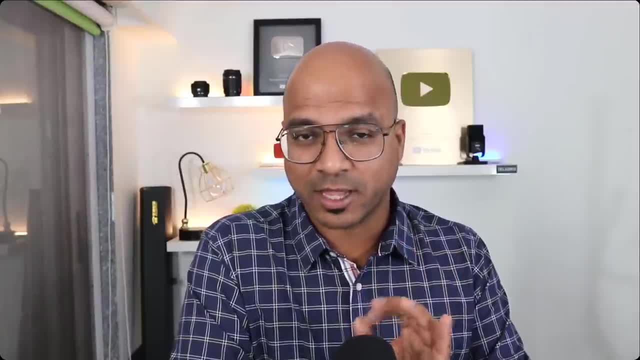 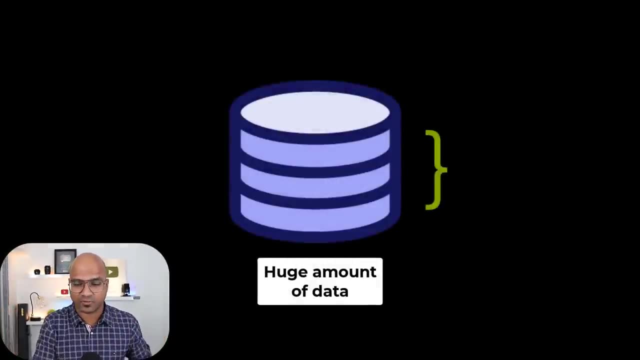 will store half data and half will be undone. so it's awesome. and also at that point you know the data storage were very costly. so they were working with this huge amount of data of kbs and they wanted to store this data somewhere. so they thought, hey, why to waste memory, right? 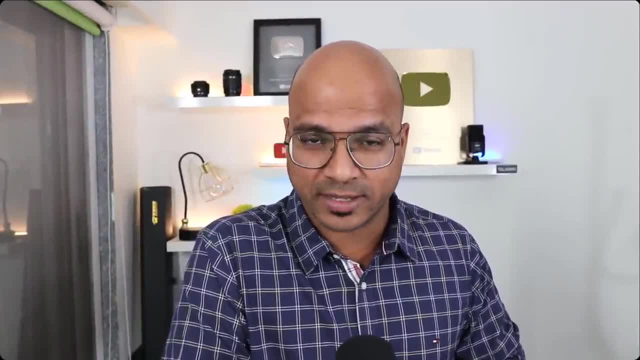 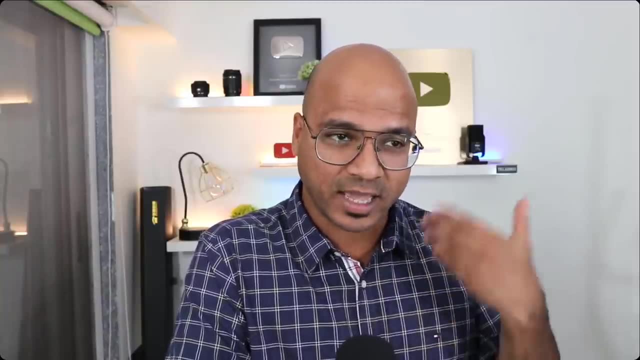 because at that time it was costly. so they wanted to make sure that every data is stored properly and there is no duplication. at least minimum duplication was there. so for that they achieved something called normalization right. so we have 1nf, 2nf, 3nf. 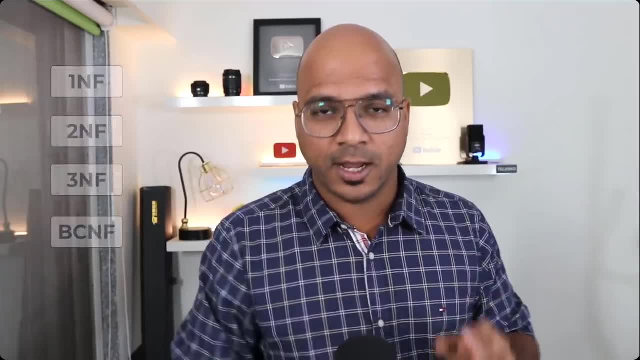 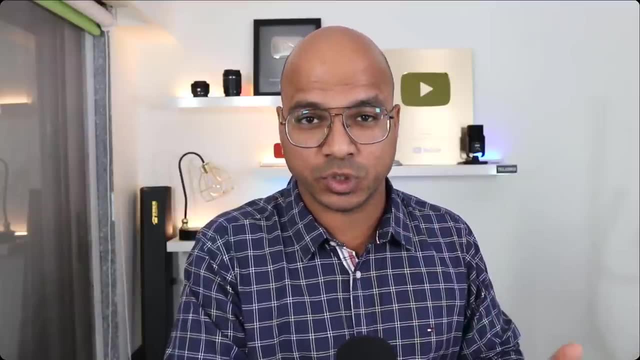 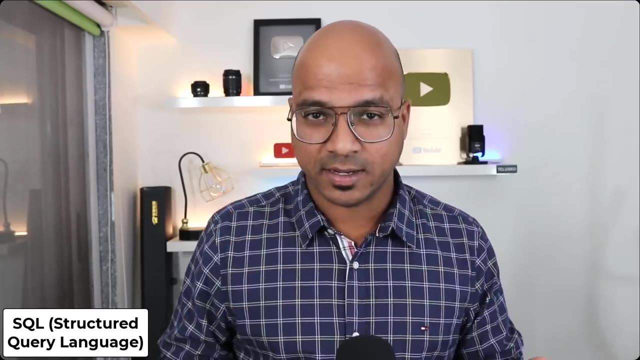 and bcnf. of course it's a huge topic to talk about, but it actually creates relation between tables and there's no duplication. that's the end product of that and it is easier to store and you can use a special language called sql, the structure query language, to fetch data. now there were different. 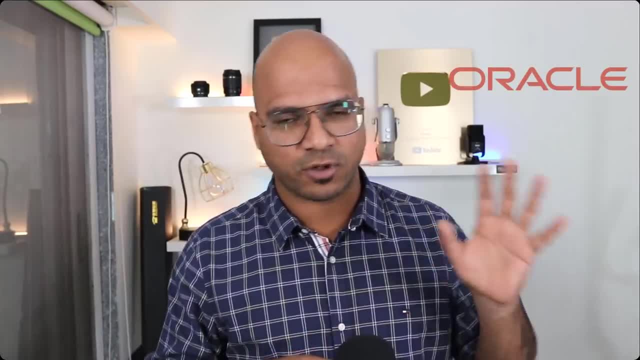 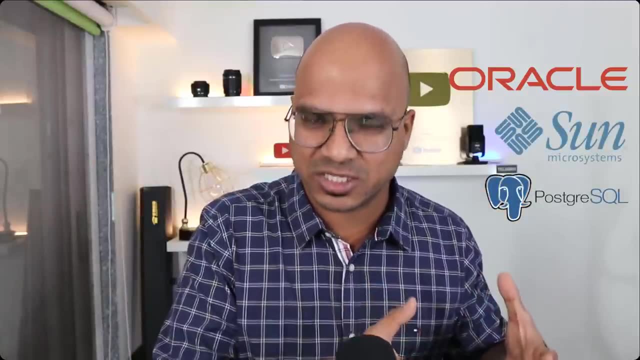 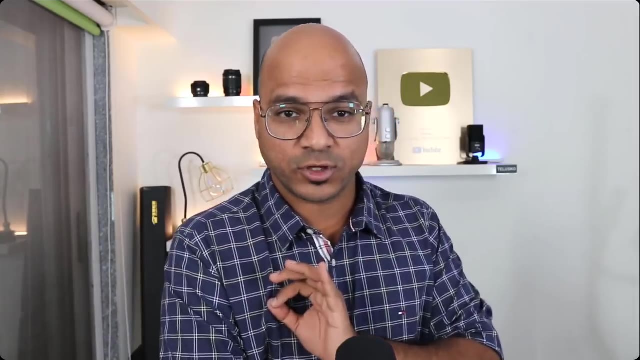 databases available in the market. we know from different companies, from oracle, from sun. then we got open source project like postgres, so everyone had their own way of implementing it and there were slight changes in the sql language, but ultimately the language is same, right with some tweaks, and it was awesome. so everyone was using sql. in fact, i started my career with sql and i 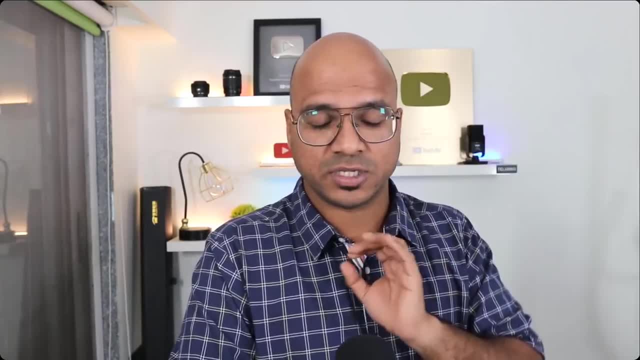 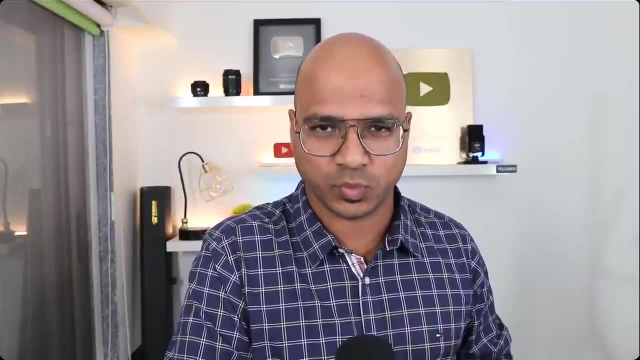 was so happy. so sql basically started around 1970s. it's a very strong language, well tested because they're from a long time. so it becomes a first choice for any database is in this world right. but then there were some issues. you know when, after year 2000, most of the 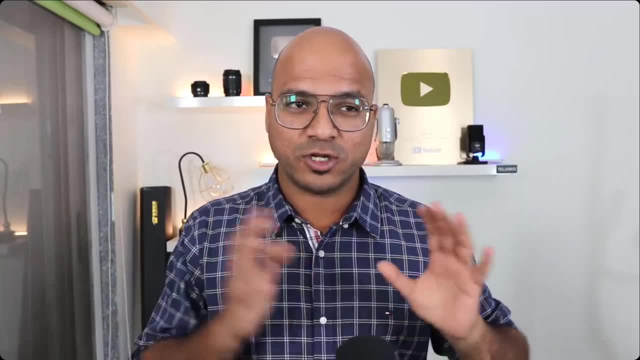 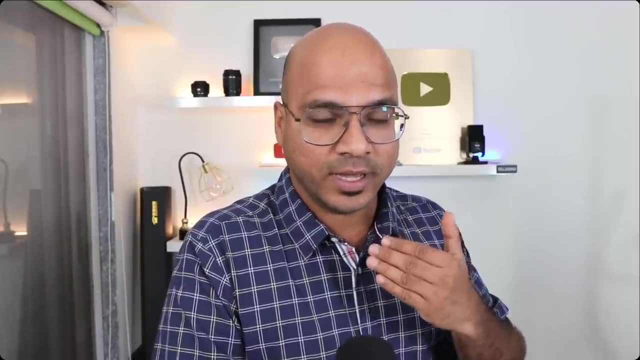 companies. they went online as web 2.0. so issue of storing data only by companies where they have structured data, instead of using only for the internal use. now the, the internet or the database system or the id in general was available for everyone even before the common public. 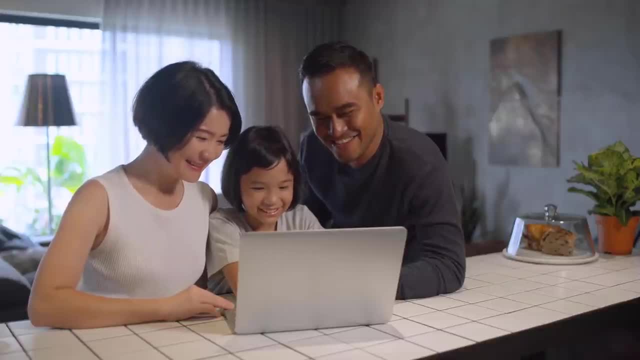 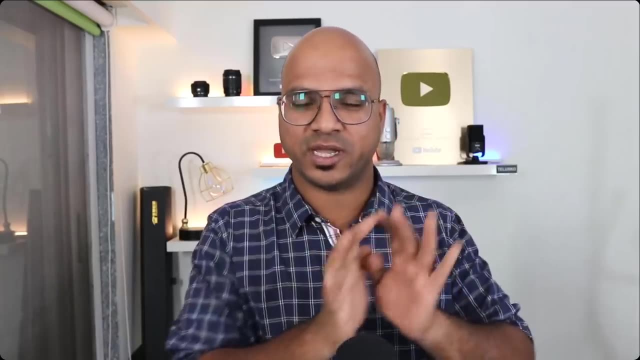 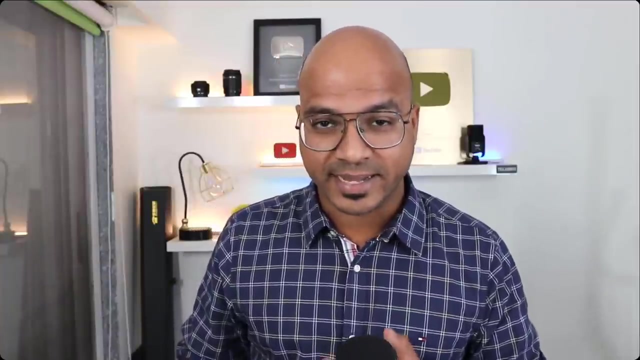 and now we wanted to expand it, not just normal data storage. we wanted to store audio video files and maybe unstructured data where you can just push your data, push your forms, now, when you have huge amount of data, and also i'm not just talking about data generated by users, data generated by 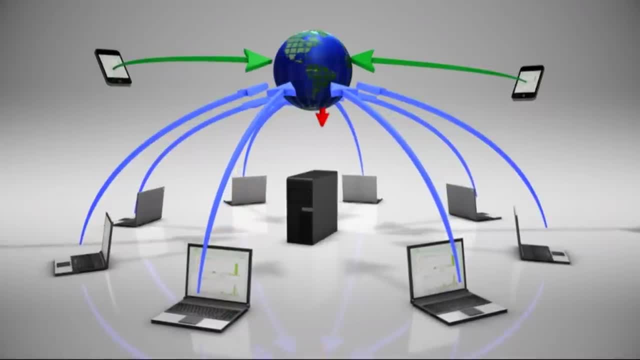 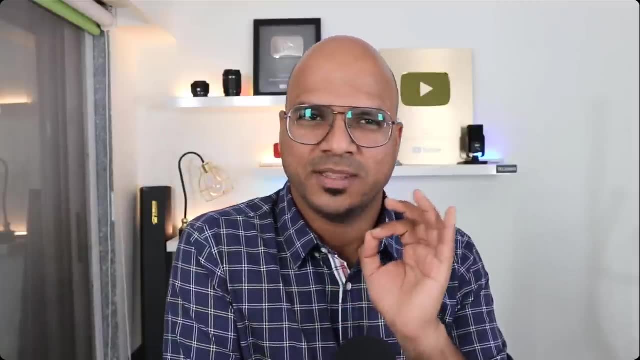 machines as well. you know, your mobile phones continuously send data to these companies, right? okay, we can talk about those things later, how they spy on you, but important thing is they are collecting data and they wanted to find a way to store the data. and also about iot devices, right? 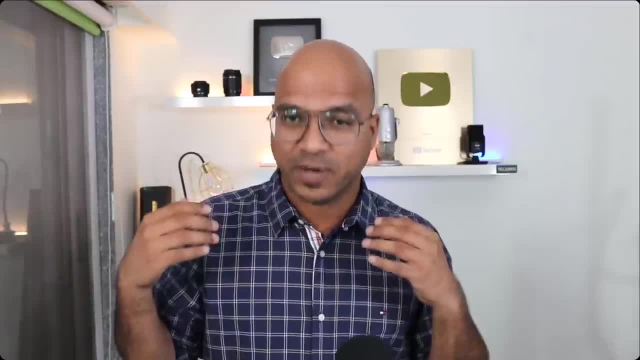 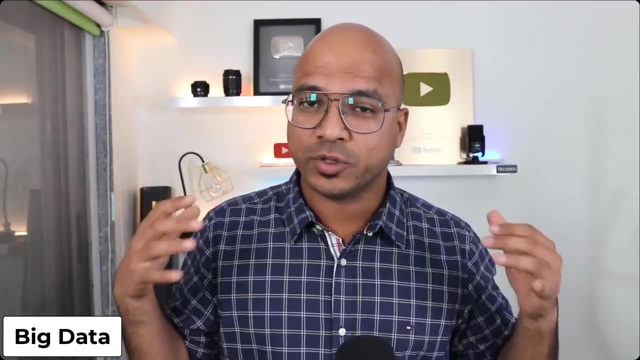 so where do you store all this data? right? we got machine learning. for machine learning, you need huge amount of data, so we got this concept of big data right somewhere around 2010. but before that they wanted to find a way, somewhere around 2000, to store data right. so they did a lot of research. 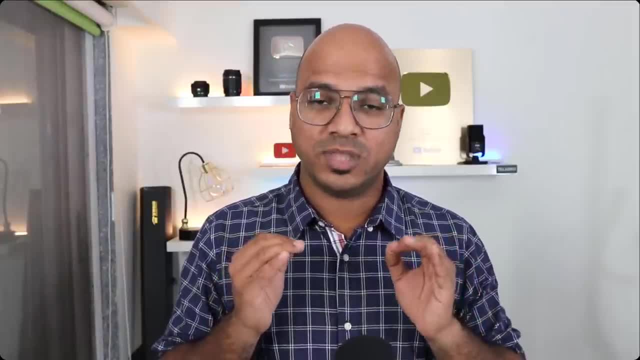 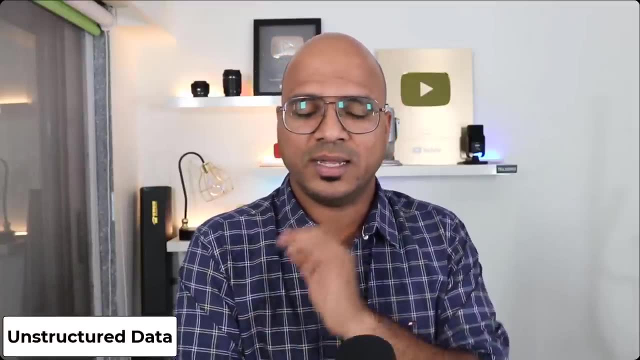 and it took them again. it takes a lot of time to build something new, right? so they came up with a solution where you can store data which is not structured. okay, there's one more thing. when it comes to structure, it's also about schema, right? what is schema is a. 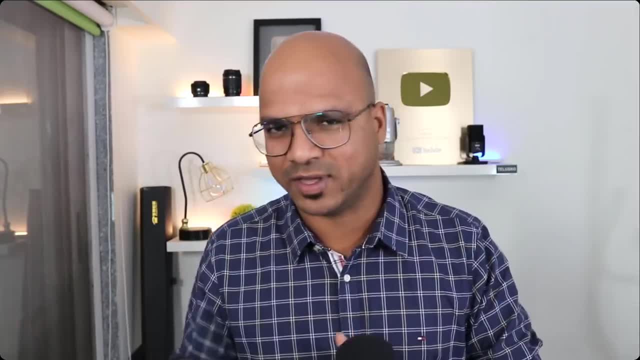 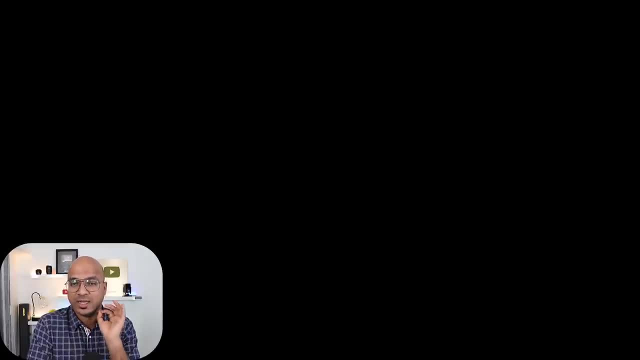 table structure, how many attributes you have and how many columns you'll be having those things. the problem is in sql. whenever you want to store data, even before you store data, you have to make sure that you have a table structure. you have a schema with you: specific columns, example, let's 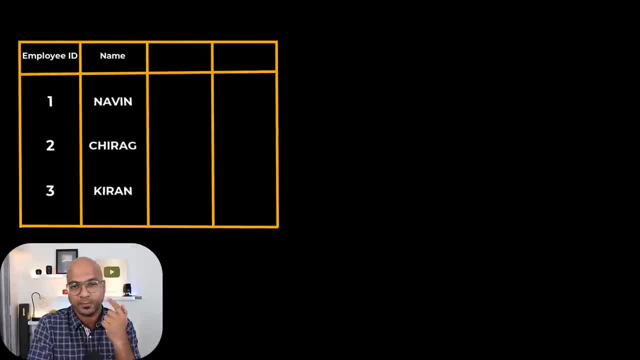 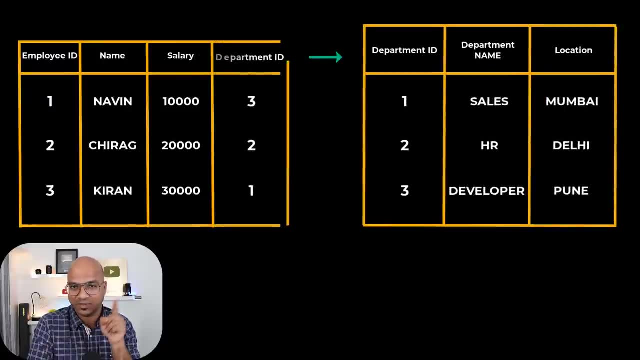 say, if we talk about employee, employee will have employee id, employee name, employee salary, employee department. yeah, if you use normalization you will be having a different table for department, but you will be having a foreign key. if you don't know sql, that was how it looks like. 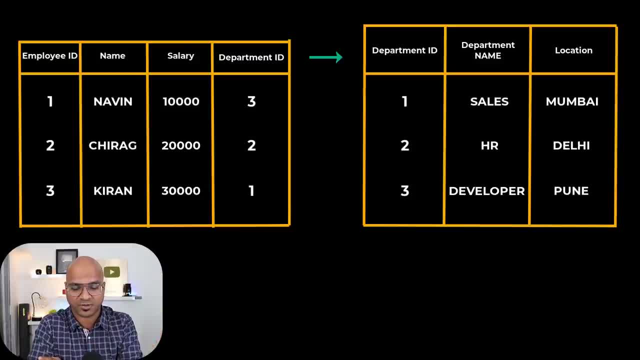 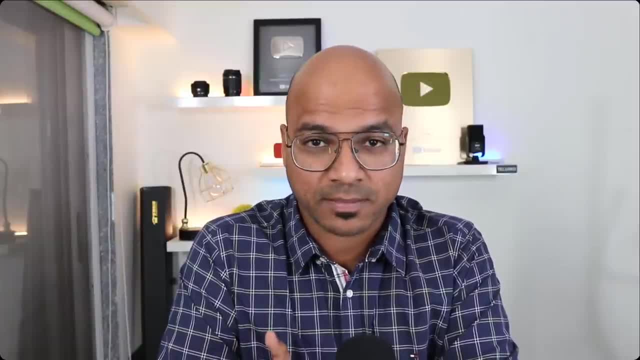 a normal table, a very simple one, actually. i'm going with a general example of sql. now the thing is, when it comes to, uh, this concept here, you need to have a schema ready, but sometime you don't know what type of data you'll be getting right. uh, that that was one issue. the second issue is about the 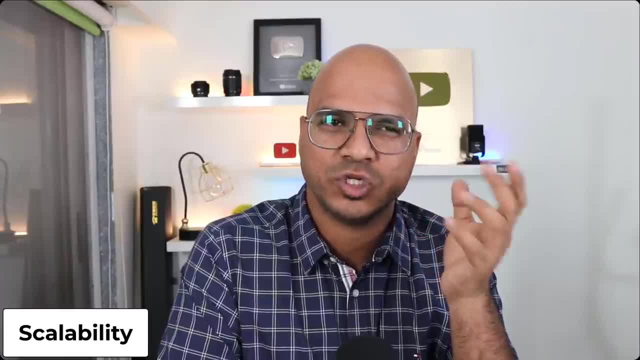 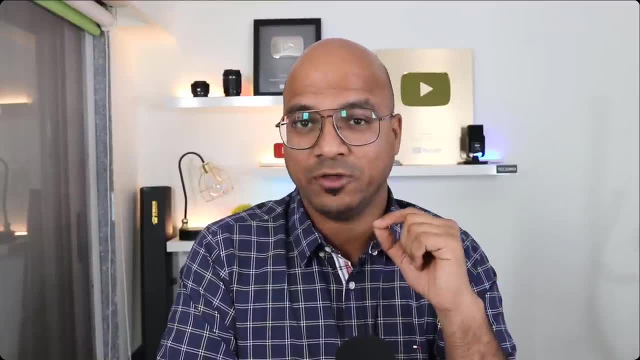 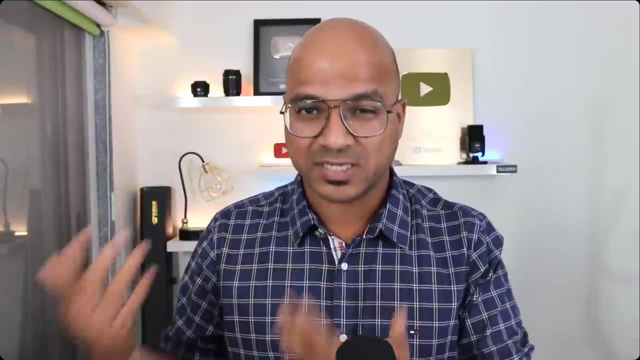 scalability. at that point, scalability was not an issue because we were having limited number of users online and they were fetching normal data, not a lot of processing required. but now, if we talk about users, we have billions of users getting visited. uh, billions of visits are happening on each website, maybe per second. there are millions of. 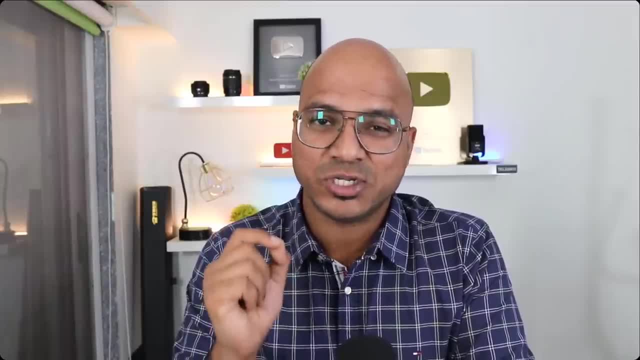 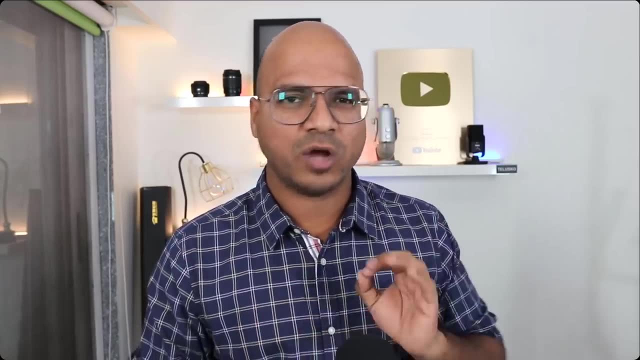 heads how they are going to handle this huge requirement, right. so they have to scale up the application. now how do you scale uh application? basically, you scale the server right. how do you scale a server? so let's say you have a normal server which has a database system, and now you 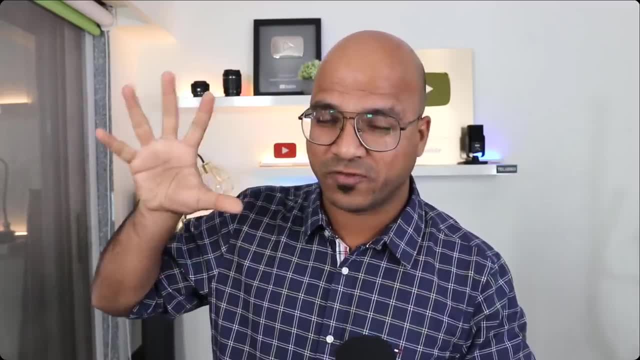 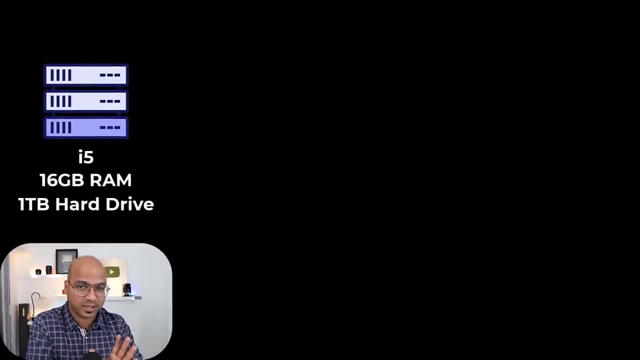 have a normal configuration. so instead of talking about all those weird configuration, let's talk about normal configuration. let's say you have a server i5, 16 gb ram, one terabyte hard drive and you have a server that's working. but now you are getting more hits. maybe you're doing some new. 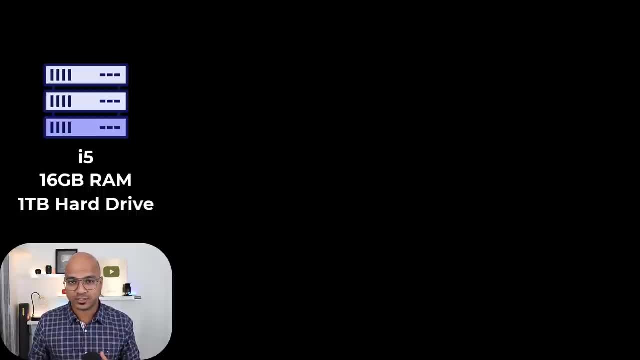 event and there are some sales going on. now you have more users, so how do you handle those users? right, you have to increase the capacity of your server. how do you do that? so, basically, you have to do vertical scaling, which is scale up basically, where you have to improve your system from i5 to 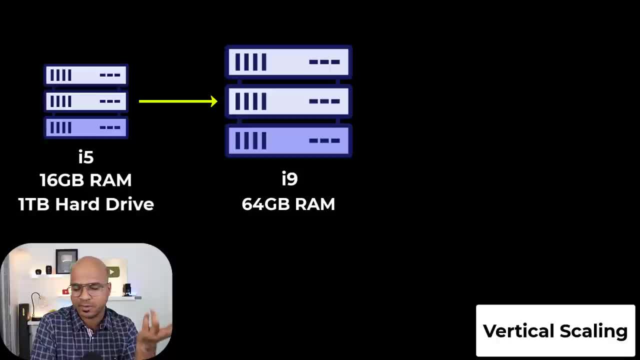 let's say, i9, from 16 gb ram to, let's say, 64 gb ram, and maybe improving hard drive as well. okay, not, that's not how you configure server, but just to keep it simple, that is vertical scaling- scaling. now the problem is, there's a limit for that. right till what point you will go, because 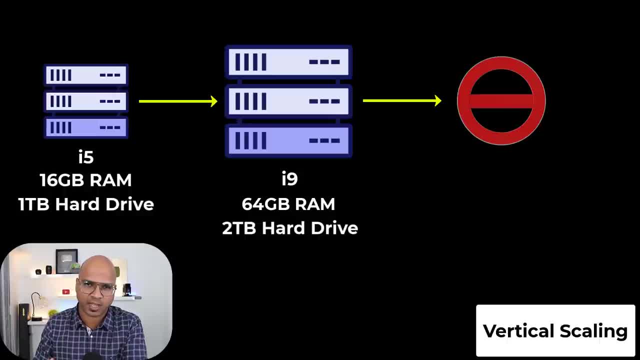 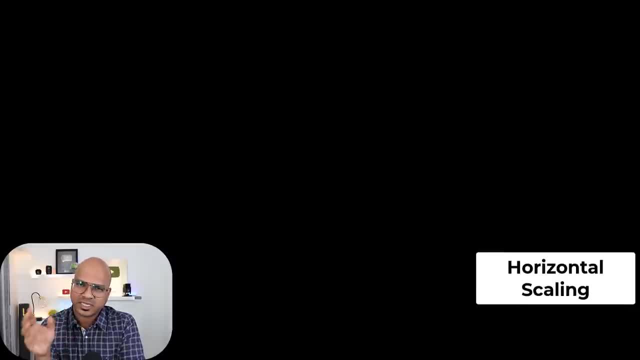 we don't have a powerful cpu, apart from i9, of course, when i'm talking about laptops. but of course we have server cpus, but there's a limit for any save, any kind of cpu. but what if you can just go for horizontal scaling where you don't? you're not depend upon one server, you can have multiple. 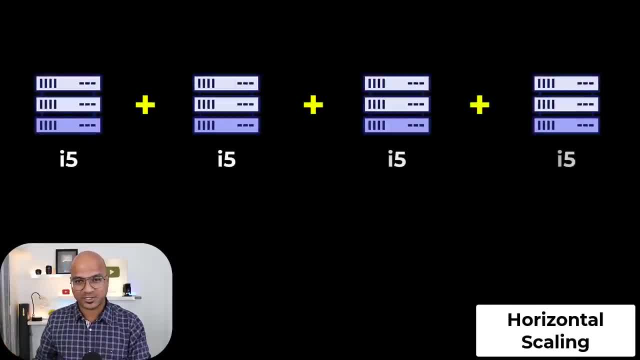 servers and small servers- right. i5, i5, i5, multiple machines- right. the advantage would be it is easier to scale because you're scaling out right. so in future, if you want more servers, just add more machines, right. it's that beautiful. so how do you solve this problem? and that's where they came. 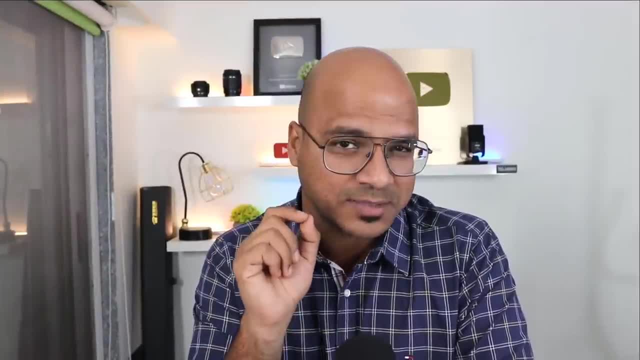 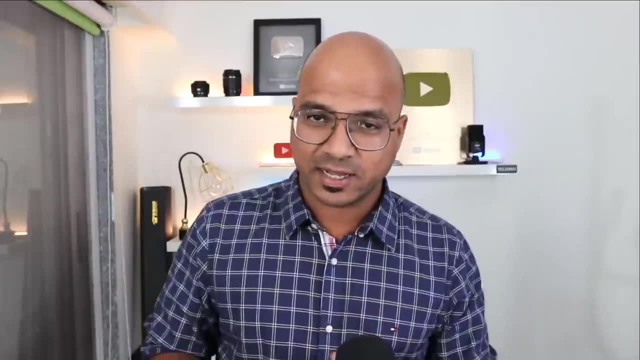 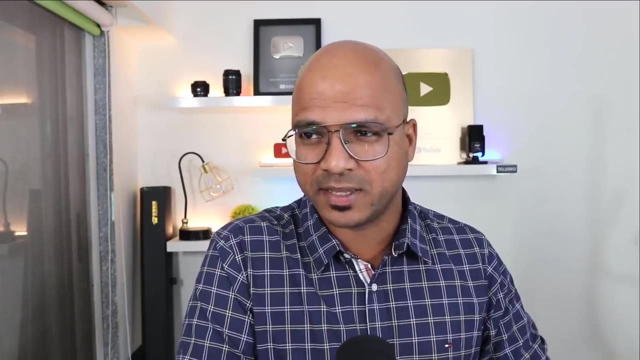 up with this technology called no sql databases. now why i'm saying databases? because we don't have one solution, we have multiple solutions. there are different types of databases available there now. basically, different companies came up with different databases there- and you can see the list here- and everyone was happy they were using their own. but then of course, we have to come on. 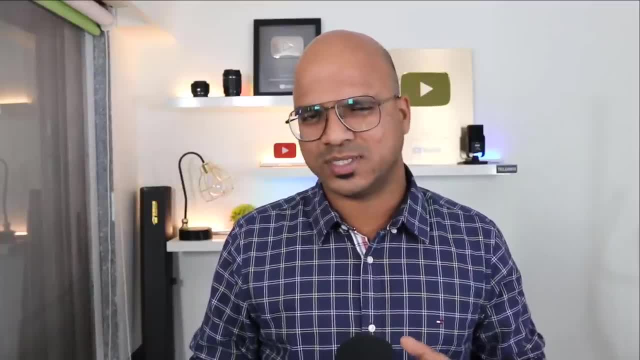 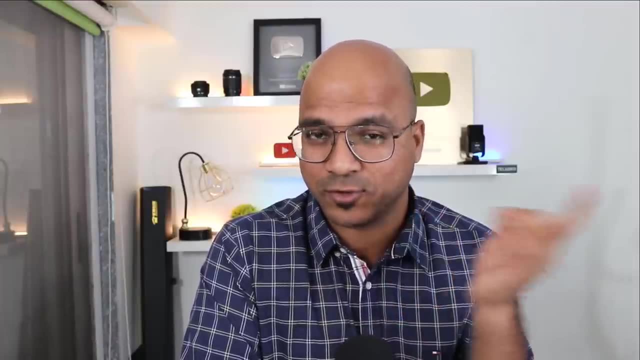 some ground right. we have to use some open source solution. so of course we got some open source there. now, by saying all those things, we missed one point here. why the name no sql? of course we mentioned it is not only sql. does that mean no sql also supports sql? and the answer is yes because initially, yes, they wanted to have a different name, like no sql, because now we don't have to use sql. but later on they figured out that sql is the best language. they have some amazing concepts and also we can use those things in our databases and that's why they said not only sql, because these databases. 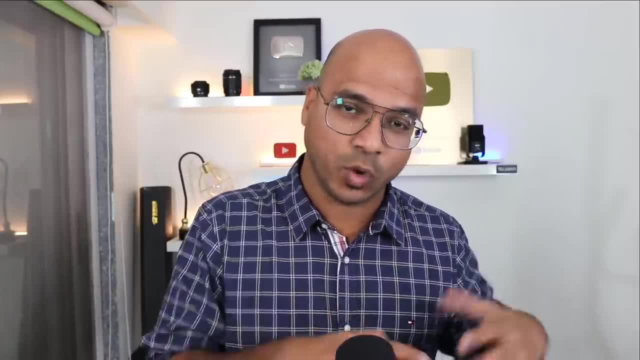 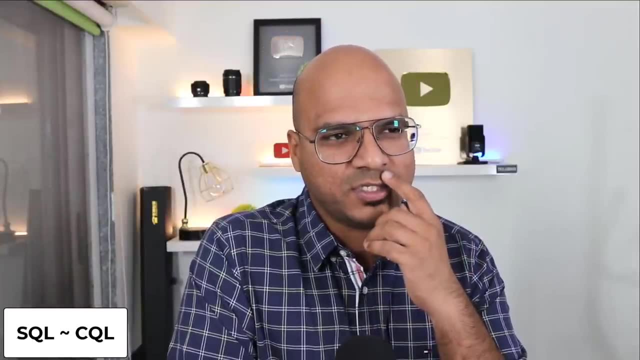 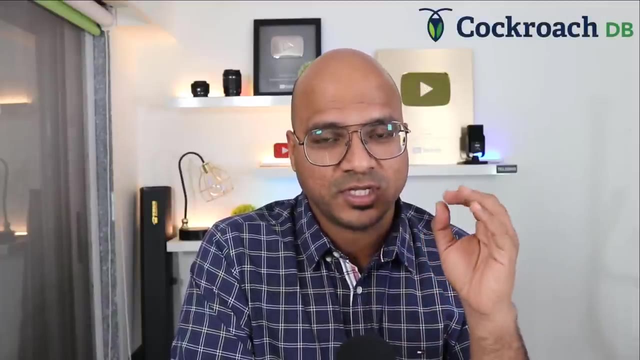 are not only sql, but also something else. in fact, few databases. they have their own sql language, like in cassandra. we have sql now. there's one more thing. if you're thinking, rdbms is not scalable horizontally or scaling out, actually nowadays we have some new technologies coming up. 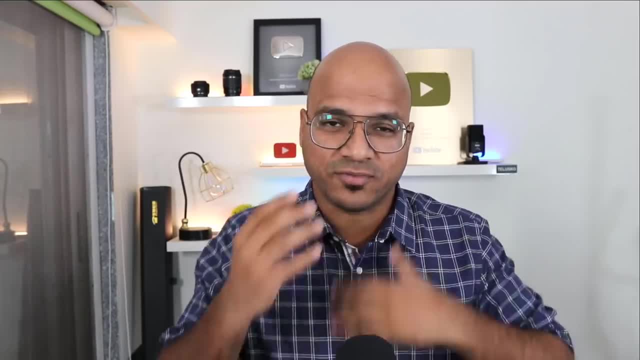 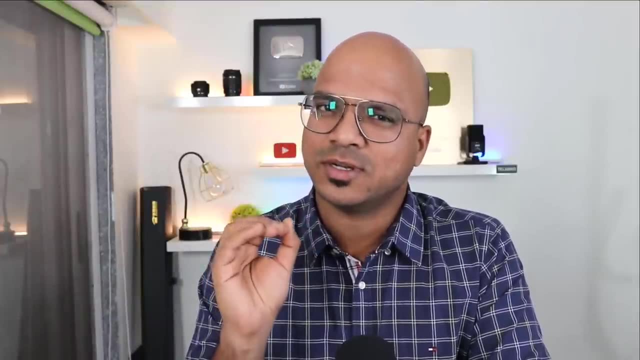 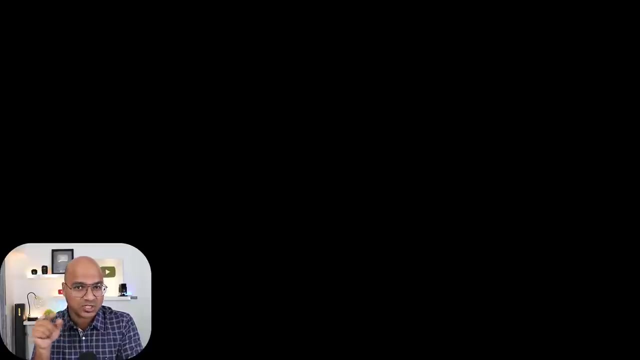 which is solving that issue as well. but then you know, that's how technology evolved, right, we have a cycle going on. so what is no sql? so basically, no sql is type of databases where it has flexible structure and it will be fast. now, why is fast? because in no sql we don't use normalization, we store data. 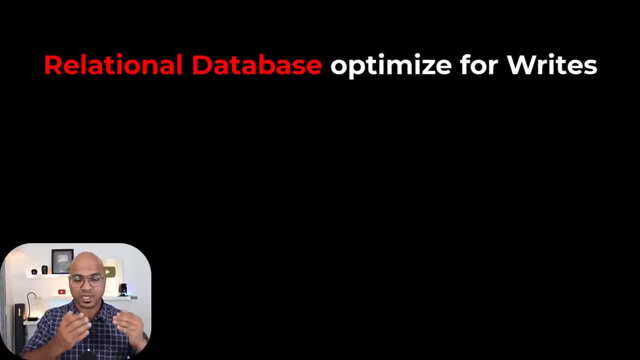 as it is right, because in sql databases the main focus is how will you store it? because we have sql to fetch data in anyhow, right, but in no sql databases the main idea is store data in such a way that it will be easier for them to access. so let's say what if you want. 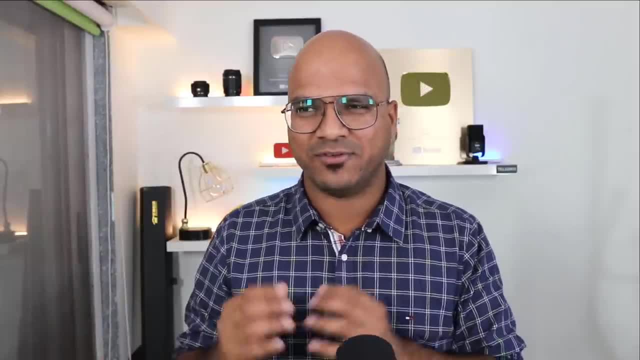 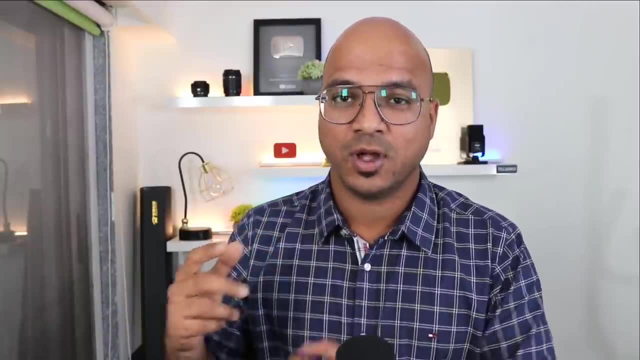 to search something, because now we don't have a normal data right. we don't have 10 rows, 20 rows, which have. we have huge amount of data to search from. so it will be easier to search, and that's why the focus is on reading, not on writing. in rdbms, the main focus was: how will you? 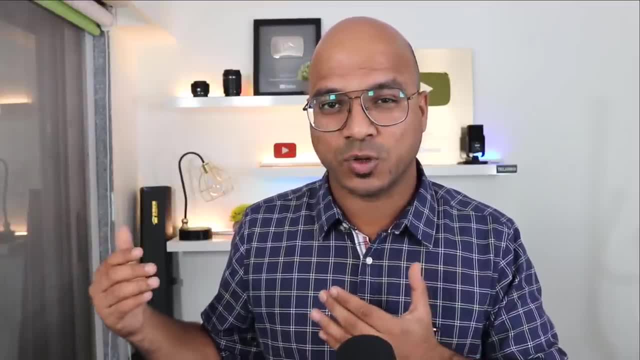 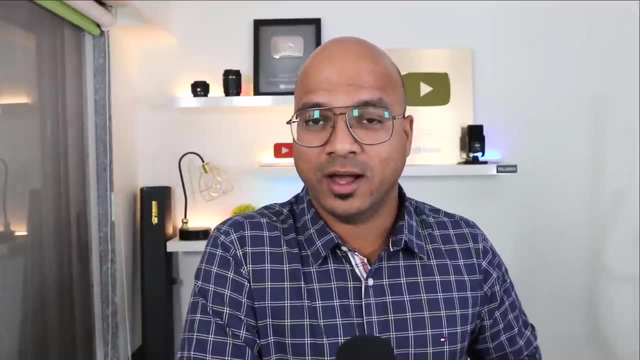 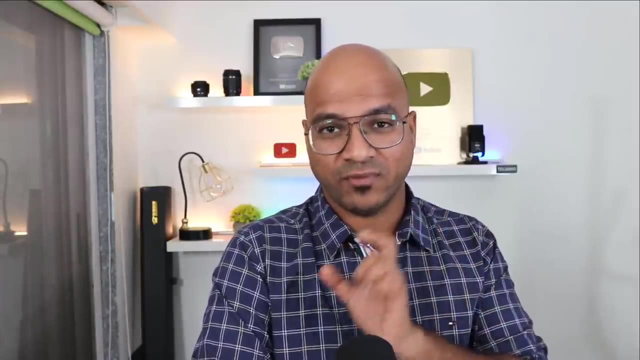 store it properly in no sql databases. the idea is to: how will you fetch it fast and easy way? so basically, we have different types of databases in no sql. uh. the first one is key value. in fact, that's the main idea of uh noise databases, right where you will be having a key and a value key. 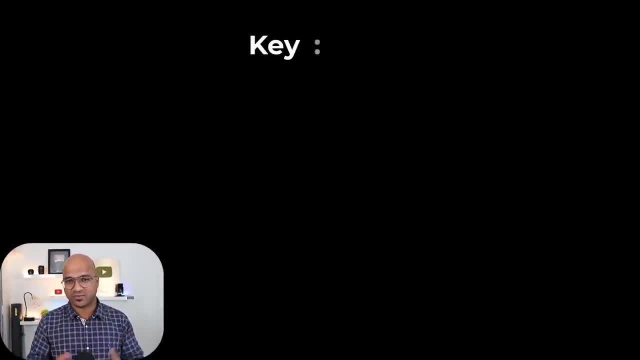 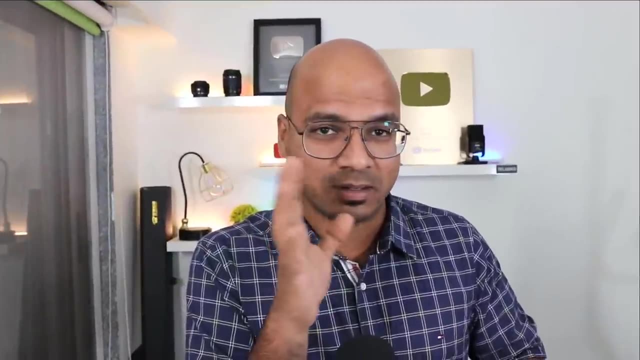 fast access. now how they do it. so let's say we have a key and we have a value, key, value, key, value, key. the thing is, you want to saying that's not what i want to store. right, it looks good for the examples, but in real life applications you have huge amount of data to store. right, that's right, this value. 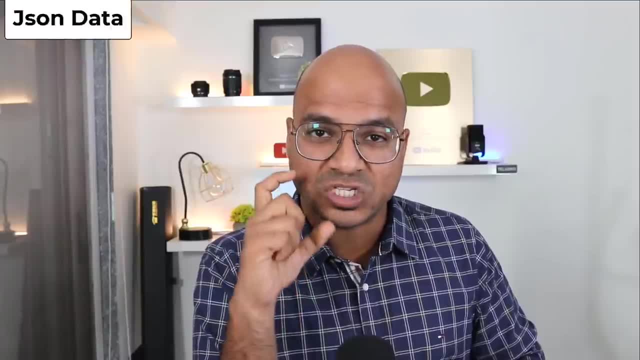 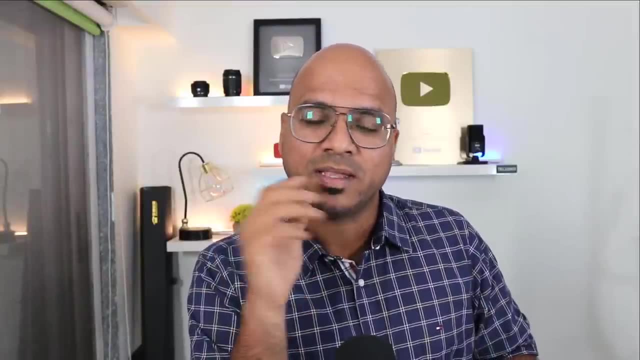 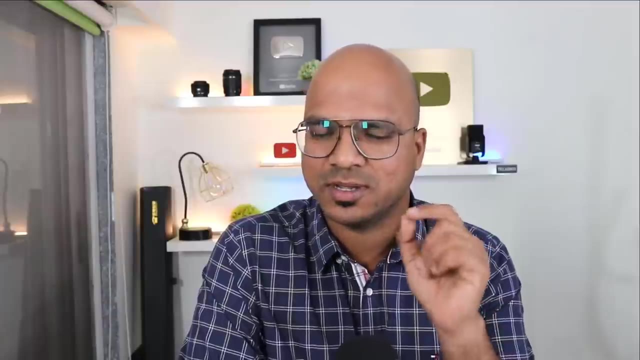 here can be a normal value. it can also be uh json data, right. it cannot. it can be anything, right. it can be multiple columns. that's your choice, right. that's the flexibility which you get, right. so you get a key value. a value can be anything. now, when i say it will be faster, it does that with the help. 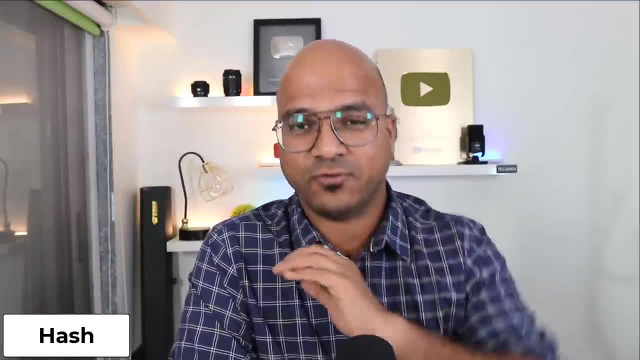 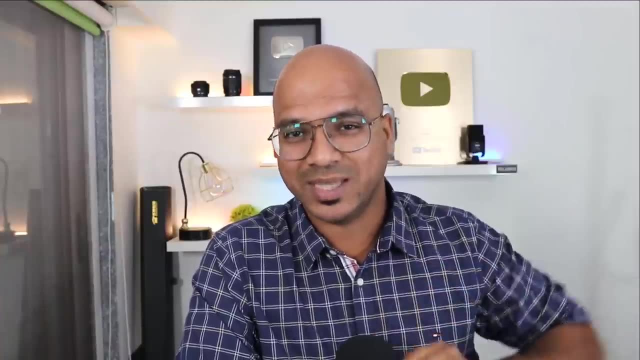 of hash, right. so if you want to search a data from millions of key values, you don't actually go in a linear format, you don't have to go for each and every row, you can simply use the hash to go to the particular point, right? that's the beauty. so that is key value. now, just because i mentioned document. 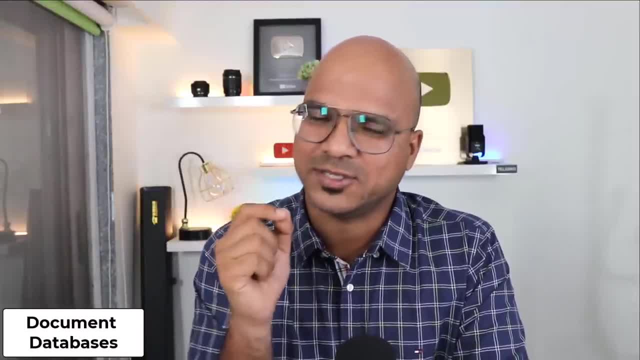 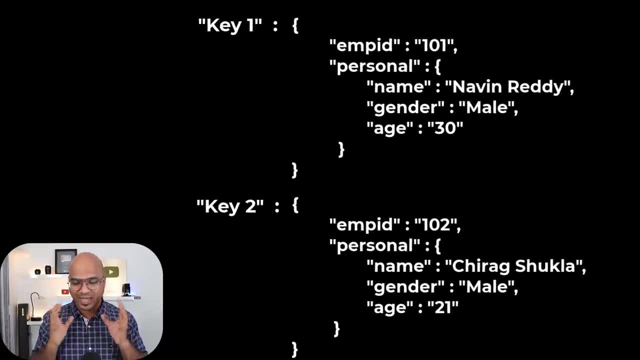 we have another type here, which is document type, or you can document databases. so here what you do is the value here is actually a json document. every time you store data, you actually store a json object in a binary format, of course, but you actually deals with json. the advantage would be: 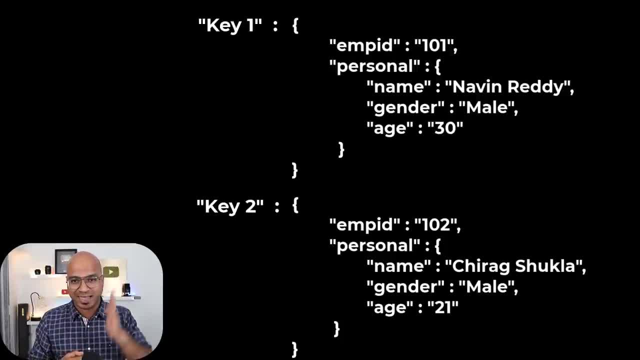 whenever you want to fetch data, you get, you got json. you send that json from the middle tier or from the server to the client right? because on the client side you'll be having, maybe, react application or android application which needs adjacent data which is directly coming from the 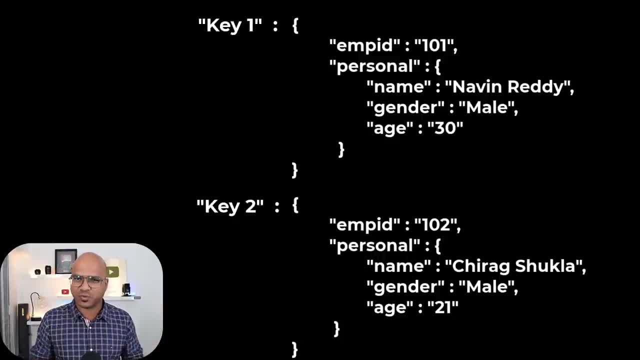 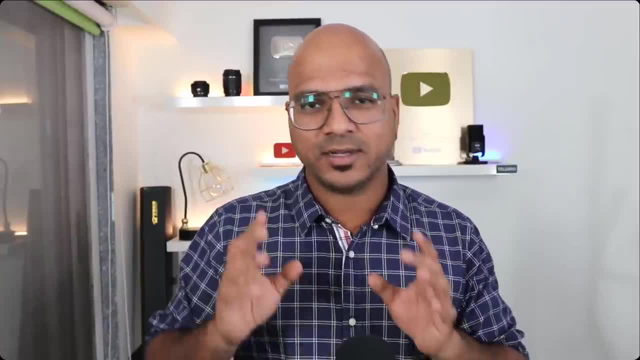 server or actually from the database. there's no processing required in between. it's so fast, right? that's the beauty, right? so that's where we have document type document databases. in fact, this is not just one video. we have series of videos coming up and we'll be explaining these. 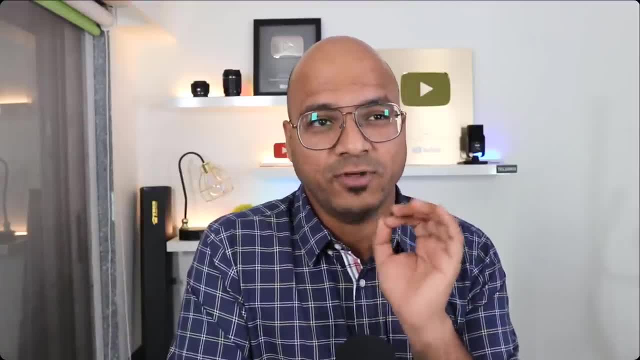 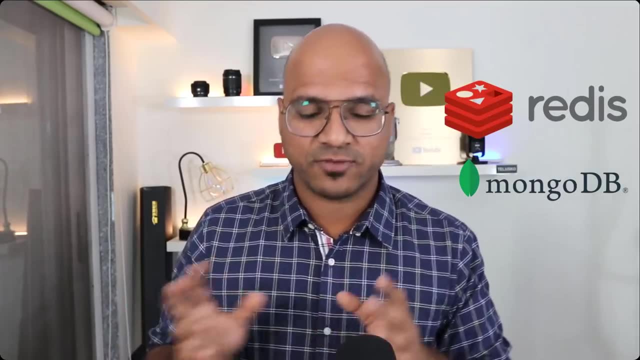 things on machine. now, since we have mentioned about the machines, uh, we will be using different softwares. so for key value, let's say, we have option of redis. document type, we have, let's say, mongodb. uh, we have two more types right for that we can. we will be using examples as well, and then 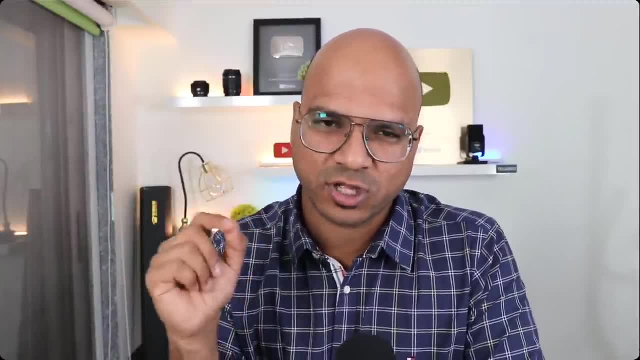 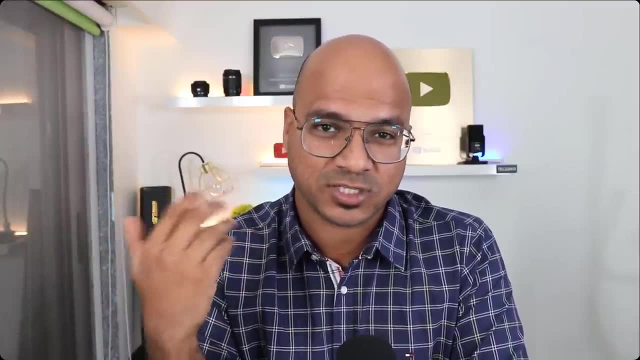 we'll be doing that on, instead of installing those softwares on your machine. i will show you the steps as well. but what if we can use a cloud service? we can directly use database service and we can create our applications there. you don't have to install software on. 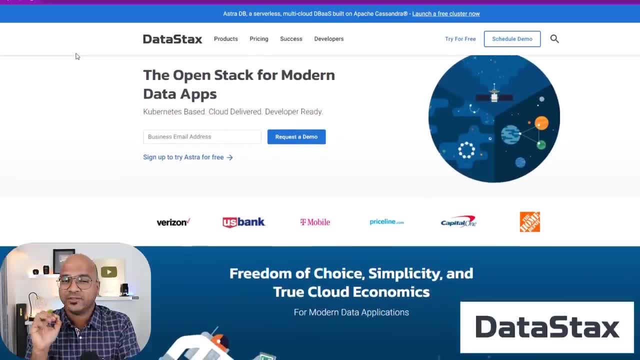 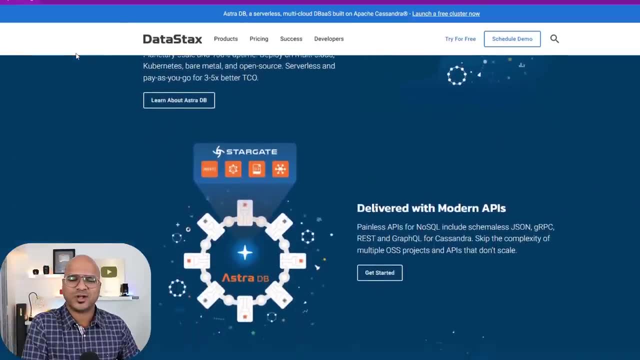 your machine, and that's where we will be using this application called data stash. in fact, the idea for this video is sponsored by data stash, so we'll be using their application because it's beautiful. so don't worry, it's not just one video. we have series of videos and we'll be explaining. 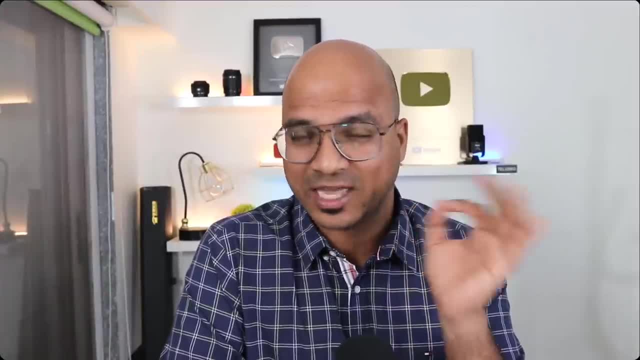 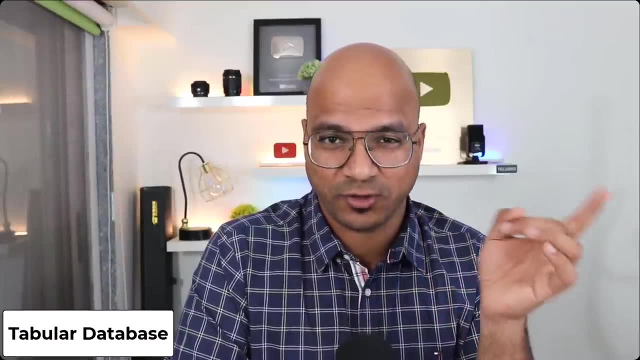 these things with examples. so we got two types right, we got key value, we got document database. in fact, we have two more. the first one is tabular databases. now i know we moved away from tables, but in rdbms and now we are talking about tables again. the thing is see, if we talk about tables. 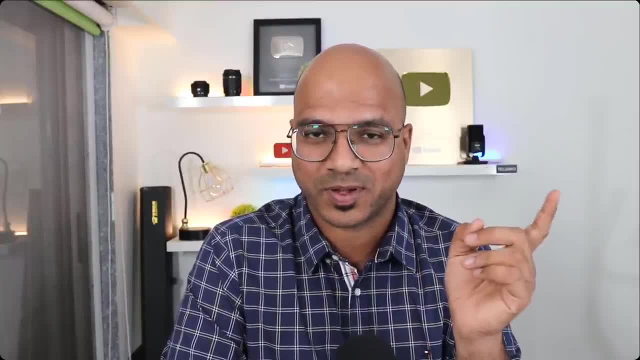 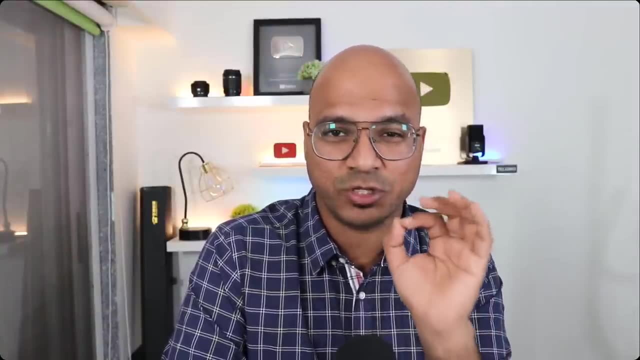 we are focusing more on columns here, not on rows. okay, so here we actually work with tables, but reverse the thing: you don't actually focus on rows, you actually focus on the columns. it will be easier to fetch. of course, we'll focus more on this in the upcoming videos. there's also a 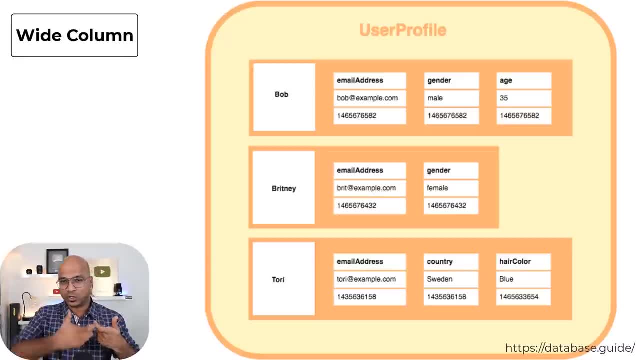 concept of wide column where you can have one key and the row and the value will have multiple columns. now it looks similar to the table formats, but the thing is, in tables we have a normal structure right: we'll be having all the columns. so if you enter a new row you have to make sure that. 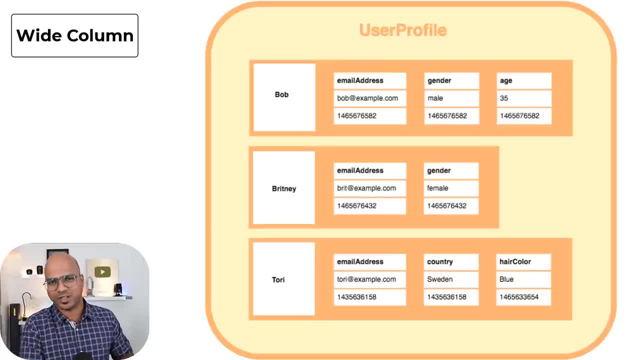 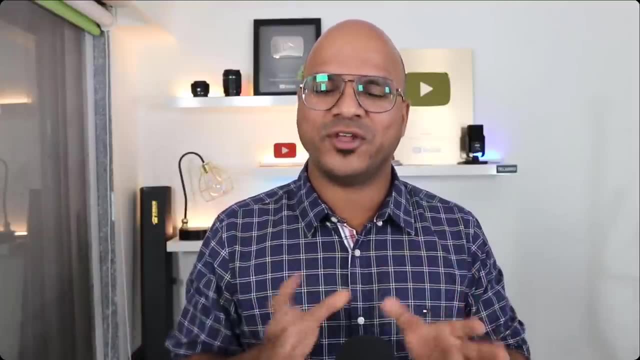 you fill all the columns. that's not compulsory in this wide column thing. only those columns will be required, based on what data you're passing. and then the fourth one: now, if we talk about all those things, know where we are talking about relations, right, but sometime you actually need a database. 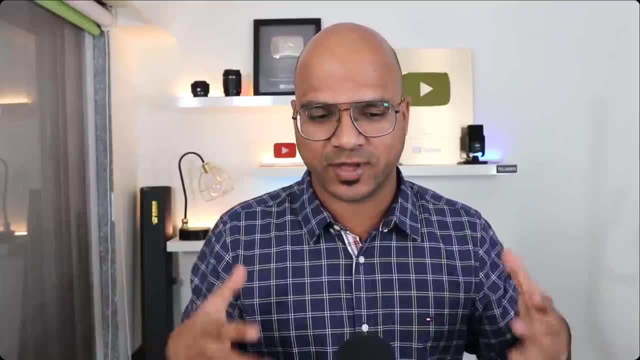 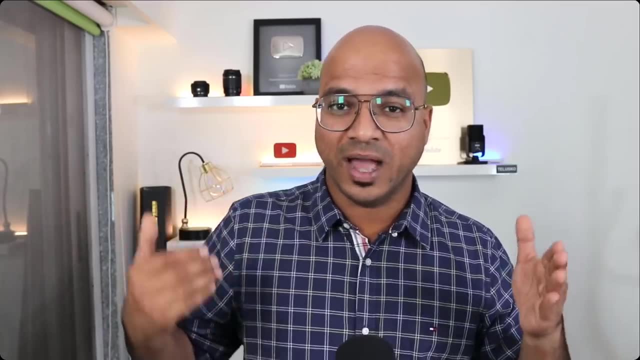 where you will find relations. think about facebook now, when you go to facebook, in fact, the next type is actually made by facebook, so they were facing this issue because they have so many users, and then we are connected. right, we have friends. so i have, let's say, 10 friends and 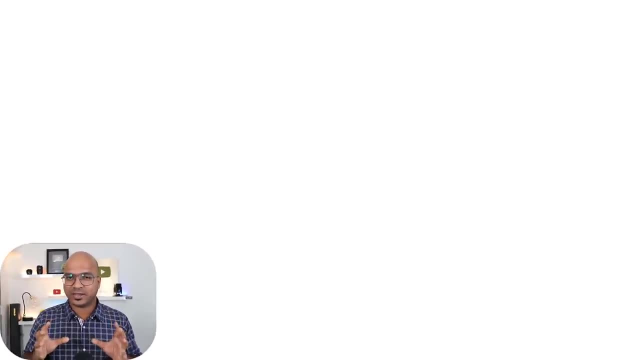 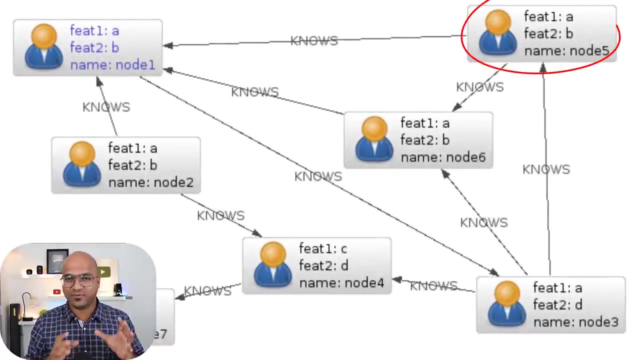 my friend will be having some 10 friends, so those are the connections. so they created something called a graph database. now graph database is actually will be having nodes and edges. every node will be like a data, like you and the relation between you and your friend is this edge, that is. 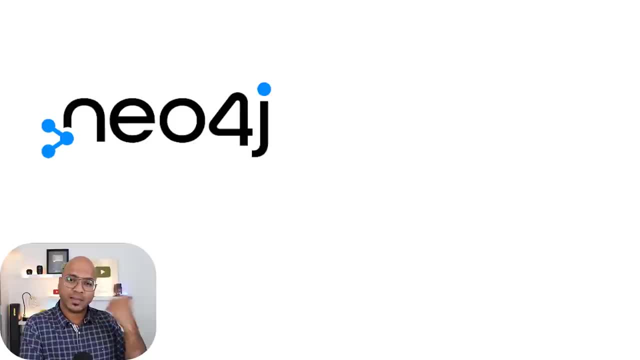 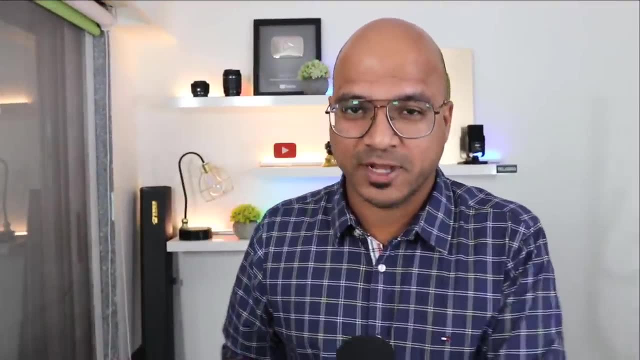 graph database, and for that we can use neo4j, and for tabular we can use cassandra. so those are the some amazing applications available to explore now. apart from this, we have one more thing coming up, which is multi-model, where you're not specific to one particular model for. 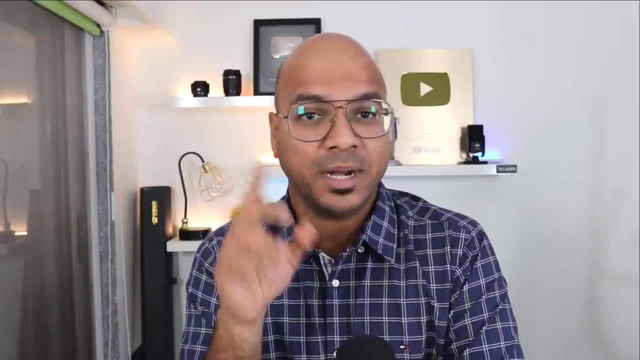 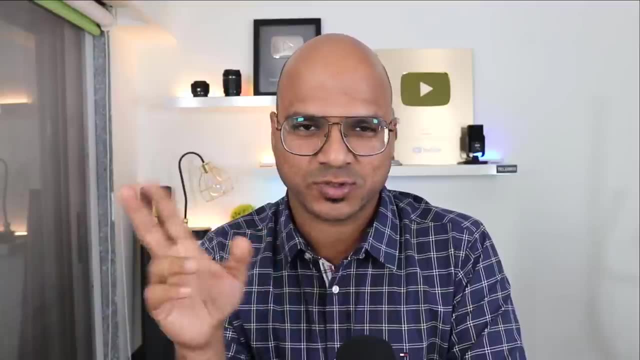 database in your application. you can use multiple models together, but the focus would be to to work on this four and we'll be using that in the examples and we'll be doing that on data stash. so you can- you can find a link for data stash. make sure that you register so that we'll be doing the.